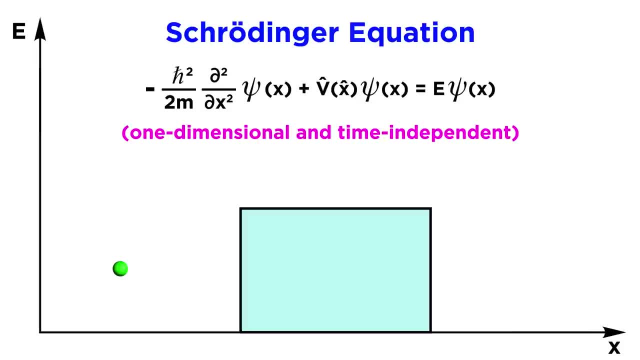 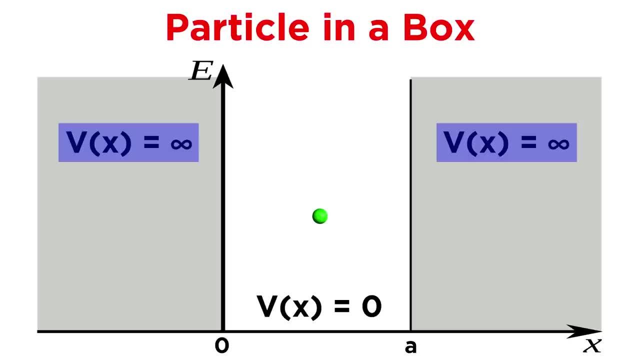 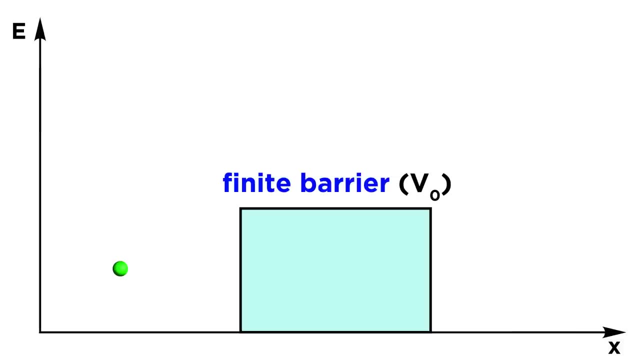 which is three-dimensional and time-dependent. Now let's quickly recall that when we were looking at the particle in a box, the particle was trapped between two infinite barriers. The difference now is that we are considering a singular, finite energy barrier, which we can refer to as v-naught, So to describe the potential in any location for our system. 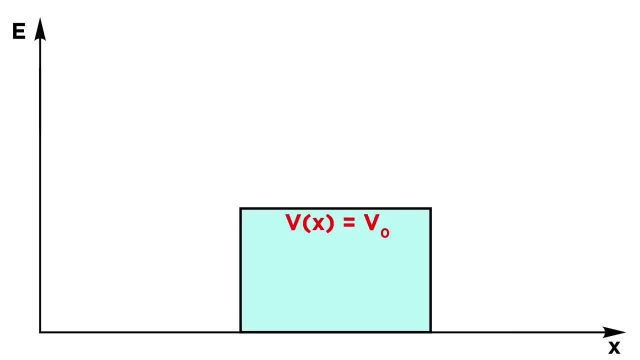 we can use the following set of equations: First, V of x equals v-naught when x is between zero and a inclusive, And V of x equals zero when x is less than zero or greater than a, which is just everywhere else. I hope you'll be able to see how that works As you can. 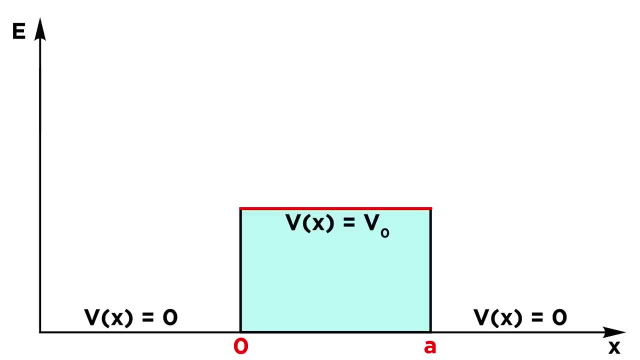 In other words, the energy barrier spans from zero to A. Now on this graph, the vertical axis represents energy. so we can see that the energy of the particle will determine whether it will encounter the barrier. If the particle has an energy that is much greater than V-naught, it will not encounter. 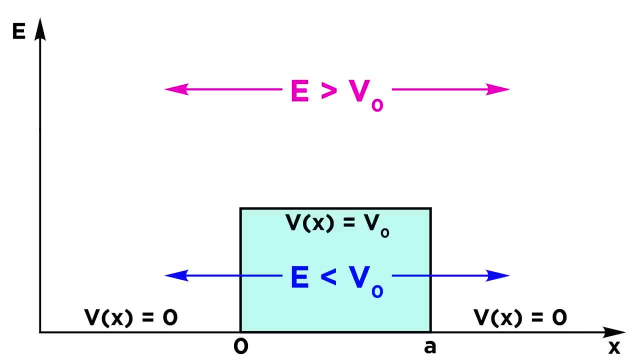 the barrier, it will pass right over it, and if it has an energy that is much smaller than V-naught, it will indeed encounter the barrier. Just to be as clear as possible, let's identify three regions on the diagram and label them: A, B and C. A is the section approaching the barrier. 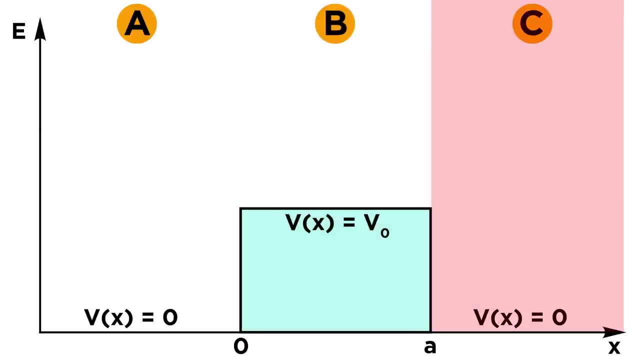 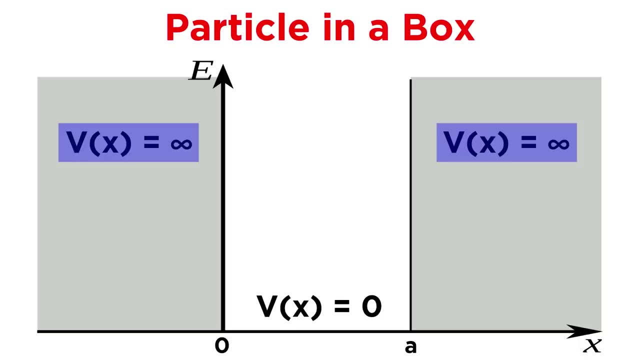 B is the section spanning the barrier, C is the section after the barrier, and any particle can have an energy that is greater than or less than V-naught. So the main difference here is that when we were looking at the particle in a box, the 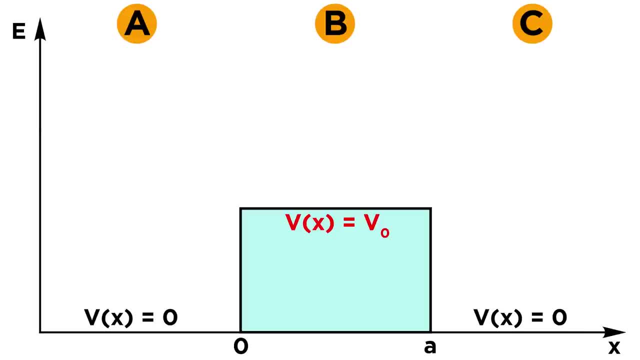 potential was infinity on either side of the well, but now we are looking at a barrier that represents a potential which is not infinite. This means that a quantum particle with enough energy- an energy larger than V-naught- can cross to the other side of the barrier, almost like jumping over a fence. 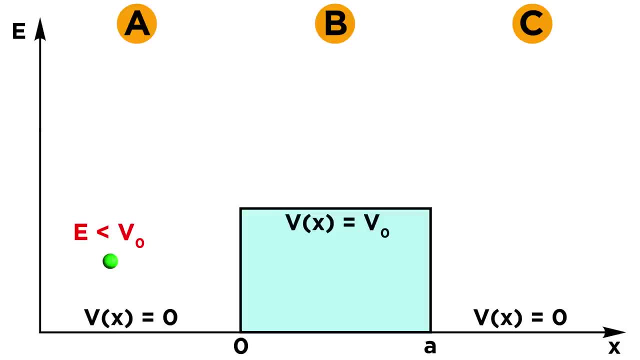 But the much more interesting situation arises when the particle has an energy that is less than V-naught. If we were thinking strictly classically, we would conclude that the particle will not be able to surpass the barrier as it does not have enough energy. 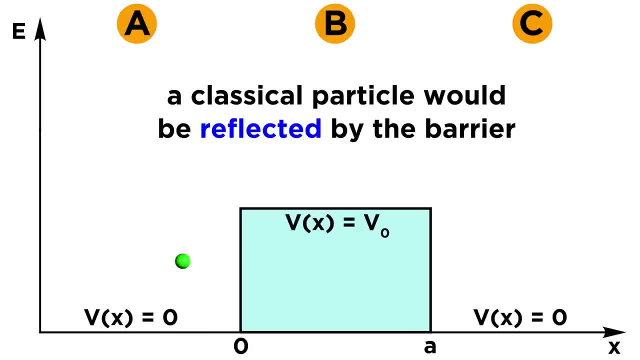 We would expect that such a particle would have a intensity greater than V-naught or smaller than V-naught, would strike the barrier and be reflected, or essentially bounce back, and we would say that there is a zero probability that the particle would be transmitted through the barrier. 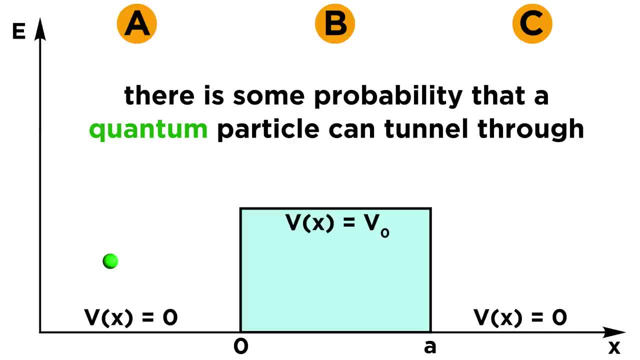 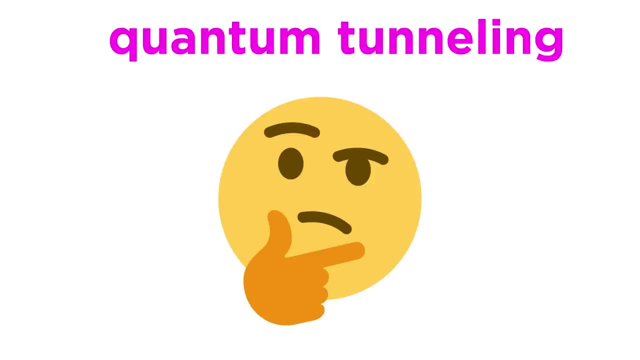 But in the quantum world there is some non-zero probability that a particle with energy less than V naught can still cross the barrier. This phenomenon is referred to as quantum tunneling. Quantum tunneling is something that is very difficult for our classically trained minds. 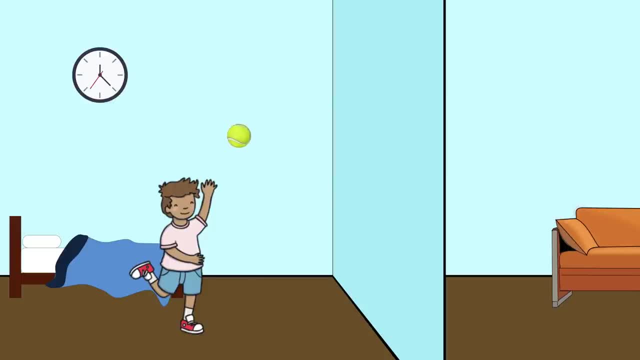 to grasp. If we were bouncing a tennis ball against the bedroom wall and it suddenly passed through the wall to end up in the next room over, we would certainly be shocked. We expect that the ball will perpetually bounce off the wall or reflect. This is what our intuition tells us must. 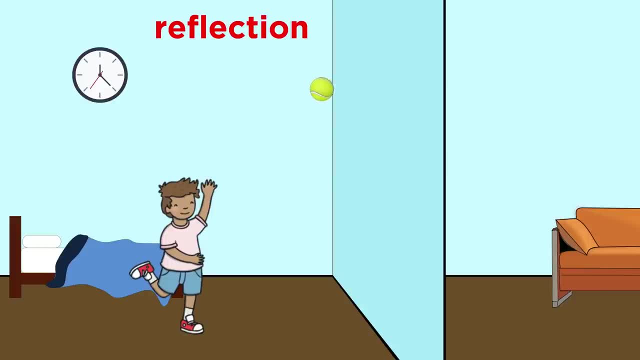 happen, But due to the wave nature of matter on the quantum level, there is indeed some probability that a quantum particle can traverse such a barrier. By the same token, if we were tossing a tennis ball over some kind of barrier, we would expect that the ball would bounce off the wall. 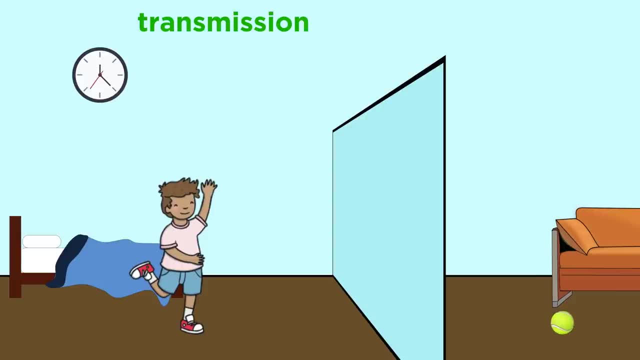 If we were tossing a tennis ball over some kind of barrier, we would expect that it will always make it to the other side. But in the quantum world, when considering a particle with an energy greater than V, naught again- there is some non-zero probability that it will be reflected. 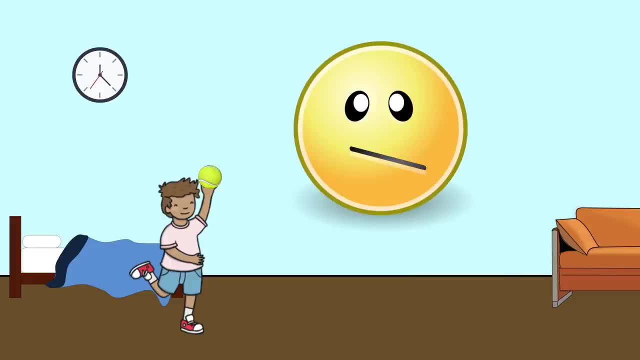 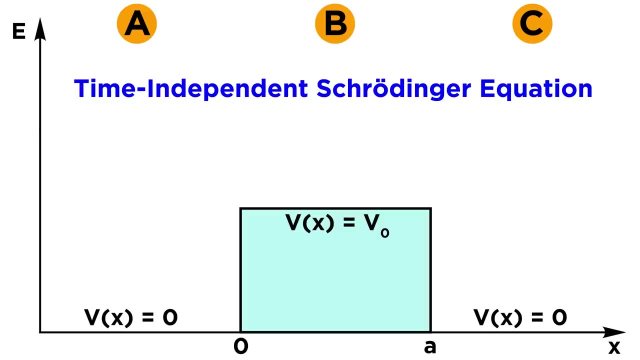 by the barrier, unable to make it over. As this all probably sounds completely insane, let's dive into the math which informs us of these facts. We are going to want to solve the time-independent Schrodinger equation for this system. Luckily, we already have. 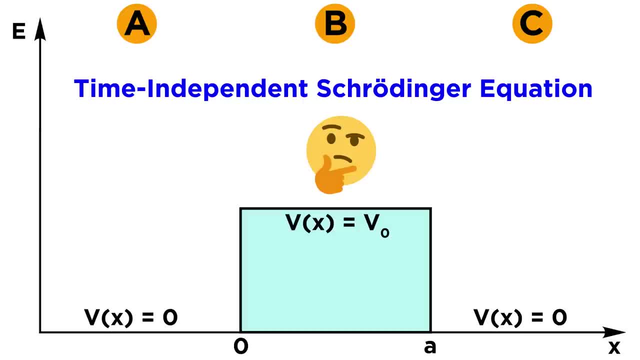 some practice with this. so if you missed the handful of tutorials before this one, make sure to watch those first. Here, we will employ precisely the same logic that we should already be familiar with. So, to refresh our memory, here is the time-independent. 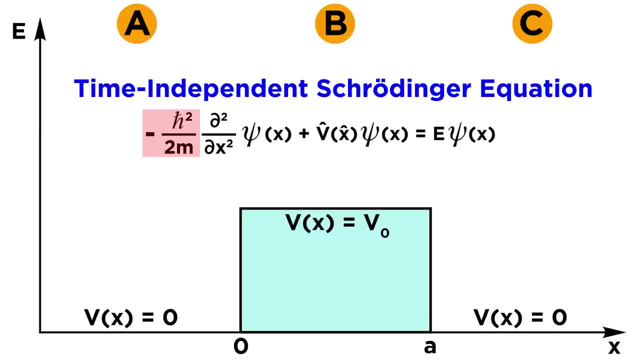 Schrodinger equation. We have negative h-bar squared over two m times the second derivative of psi of x with respect to x plus V times psi of x equals energy E times psi of x. Now, just as we did for the particle in a box, we are going to solve this equation. 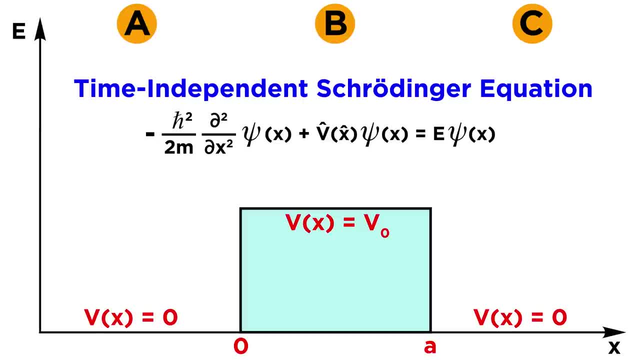 by taking into account the specific boundary conditions defined by V of x, And the first few things we will do to manipulate this equation are precisely the same as we did for the particle in the box as well. Let's begin with sections A and C. In these regions, the particle can move freely. 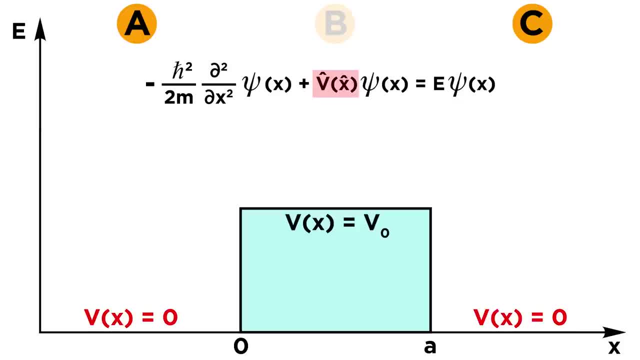 and thus can be treated just like the particle in the box, which means that V of x equals zero, and we can get rid of this second term. From here. we will take the same steps as we did for the particle in a box. We want to isolate this second partial derivative so we can multiply. 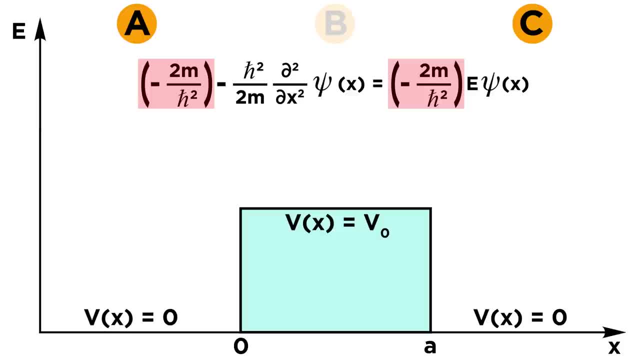 both sides by negative two m over h-bar squared, and then we can introduce the value k, which is equal to root two m E over h-bar, though in this case we will refer to it as k-naught, because this means that k-naught squared is two m E over h-bar squared, and we can make the relevant 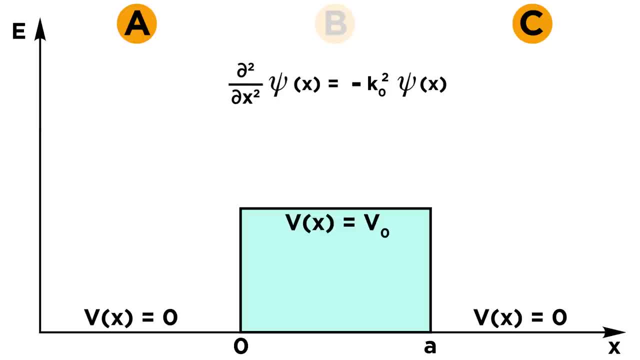 substitution. so the right side of the equation becomes negative k-naught squared psi. We can move the k term to the other side and that leaves us with precisely the same second order differential equation to solve, as with the particle in the box. In that tutorial we simply revealed the solution. 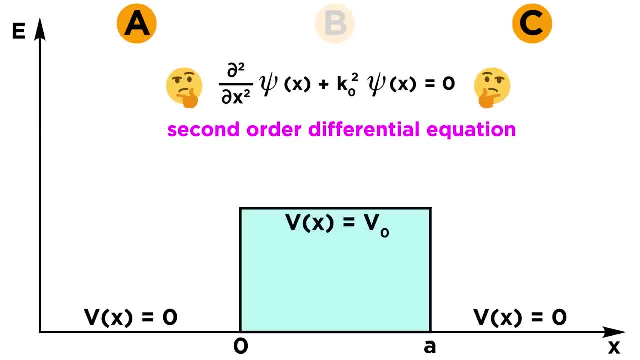 rather than rigorously. So here we will do the same thing, and the only reason we don't get precisely the same solution as with the particle in the box is that the boundary conditions are different. We are not bounded on both sides. In this case, the wave is not rigidly constrained in place. 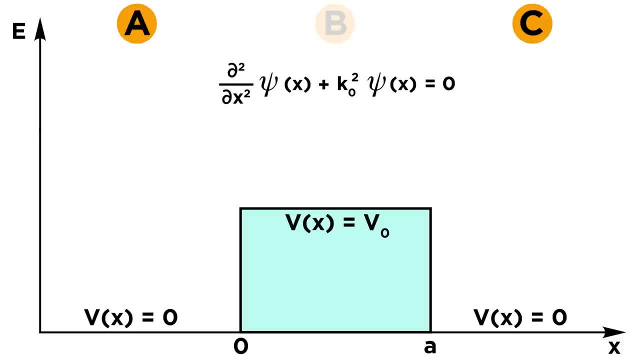 So for general help in solving second order differential equations, visit the mathematics playlist. Otherwise we can solve for psi A and psi C, which correspond to regions A and C, and we get the following expressions: So that was fairly straightforward. but now let's move on to the central region B. 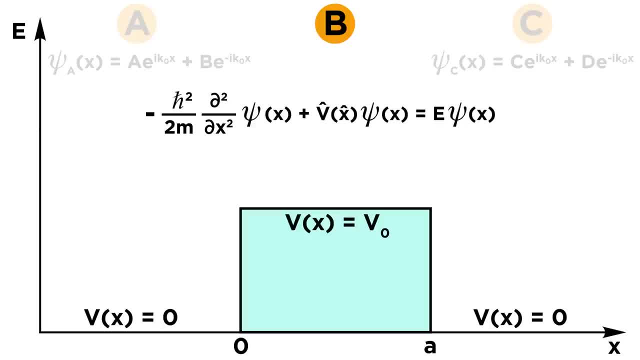 which will be a bit more complicated. Again, we can start with the time-independent Schrodinger equation, But this time the simplification we made in getting rid of the second term will not be possible, since the particle is not moving freely like it. 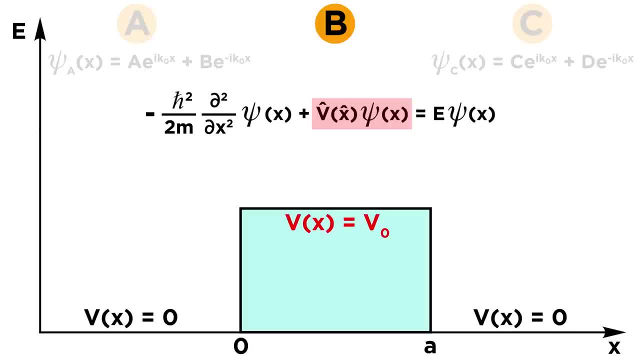 was in the square. well, We have a barrier to deal with. We have a barrier to deal with. The barrier potential will default to the second term. I think this is a strange explanation, because in this case, the particle is not moving freely. 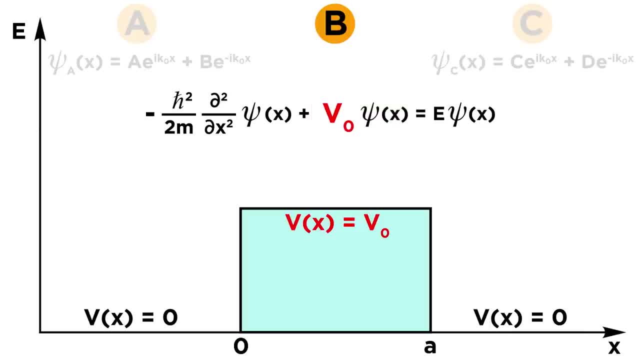 like it was in the square. well, We have a barrier to deal with. The barrier potential will not be a sign that it is a sign that it is a square. well, The particle is moving freely and the second term is drawing. the potential is represented by V-naught, so let's put that in there instead of V of X. 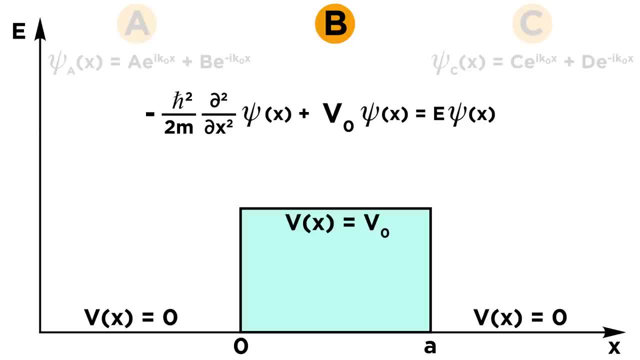 Now, in this case, we have to be mindful of the particle's energy. If the particle has an energy that is less than V-naught, the energy is lower than the barrier height and can thus be thought of as being inside the barrier. Again, this sounds like it should be impossible, but we must always be mindful of the wave-like. 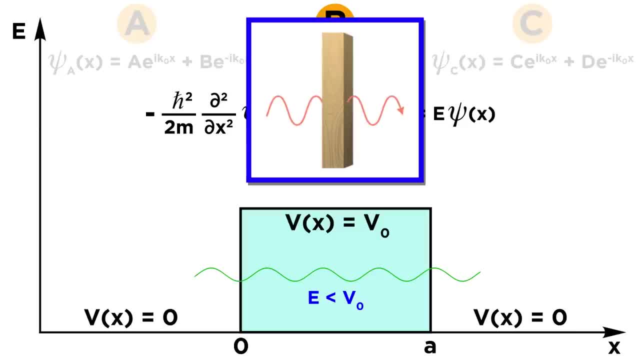 properties of the particle, Waves can go through walls, be they sound waves or the wifi you're using right now. A quantum particle can also tunnel through a barrier, and the point of this exercise is to examine what the wave function looks like when it encounters a barrier like this. 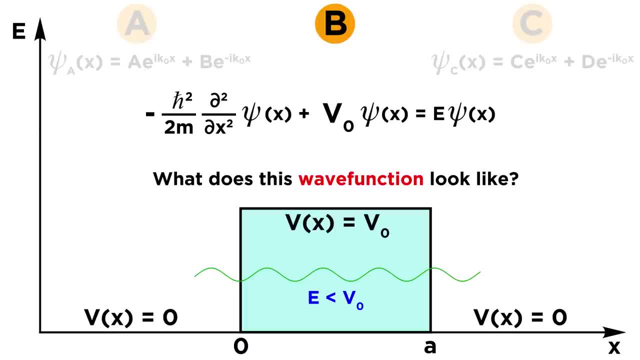 It won't be like that of a freely traveling wave, because the situation is different, so we have to do some work to find out what it does look like Mathematically. this means we can't use the same type of functions that we used when. 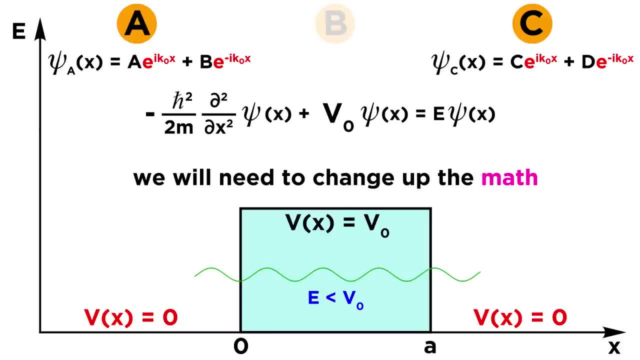 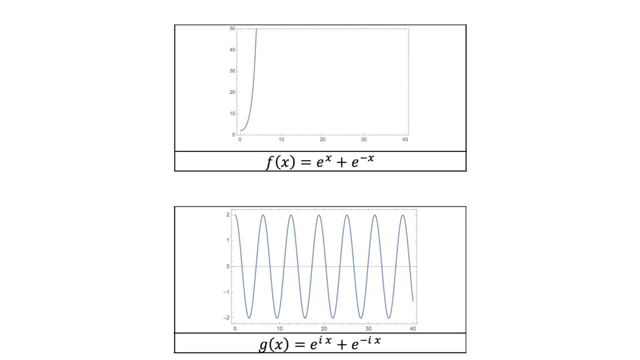 the potential was zero, which turned out to be complex exponentials. Now we must use real exponentials. Let's justify this graphically. Here we can see two functions plotted. The first, F of X, is a sum of two real exponentials: E to the X and E to the negative X. 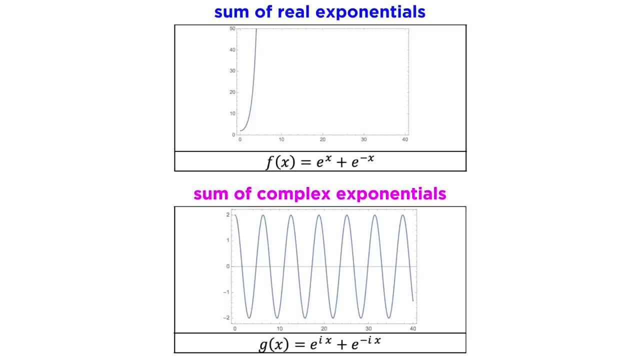 The second G of X is a sum of two complex exponentials: E to the I X and E to the negative I X. You know how G of X works because the wave functions we've encountered so far have taken this form. 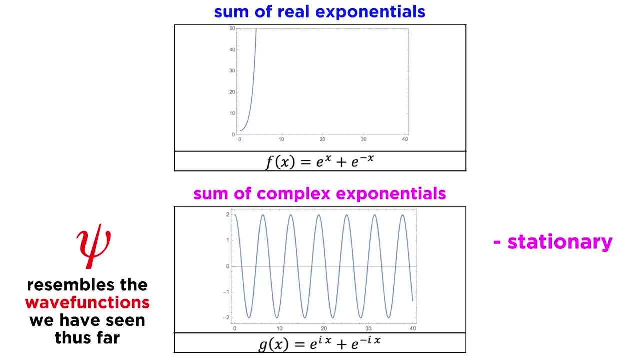 This function describes the behavior of a wave that is stationary and unaltered by a potential. In contrast, F of X is a localized function. It represents a wave that occupies only a narrow domain and then stops abruptly. This is what we will use for the wave function in section B, because it is the mathematical 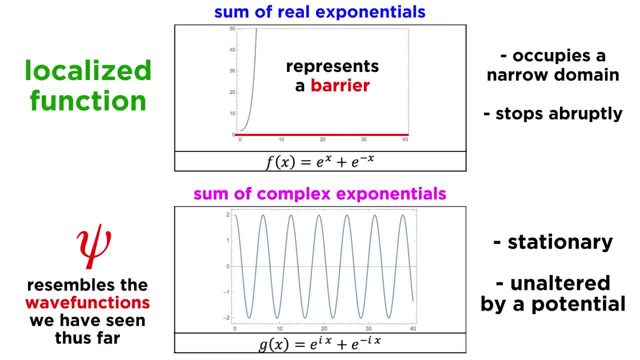 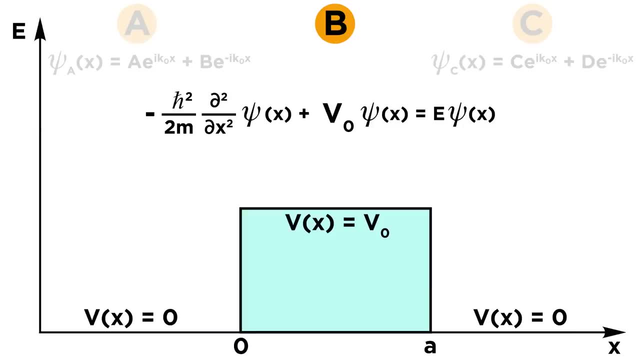 representation of the wave function. So let's look at the wave function in section B. The particle has some small chance of entering the barrier until reaching some penetration depth. The probability density function will attenuate as the particle's position distribution reaches deeper into the barrier. 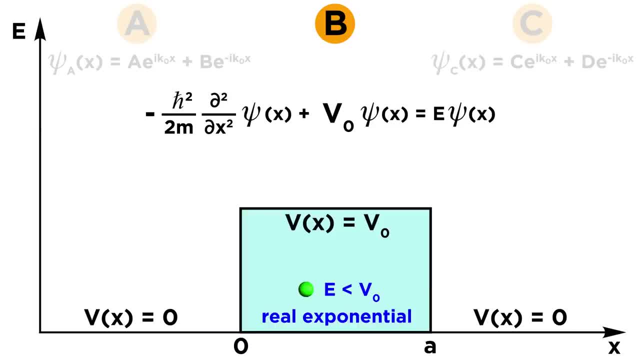 So to summarize the main takeaway here, when the particle has an energy that is smaller than the height of the barrier V-naught, we will use a real exponential, and when the particle has an energy that is larger than the height of the barrier, we will use a real. 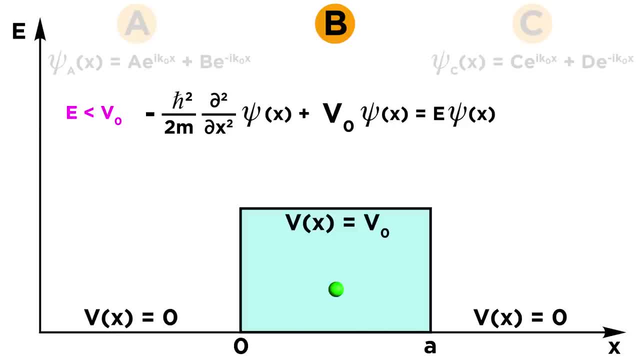 exponential. Let's first consider the case where E is less than V-naught or lower than the barrier height. Here is our equation, and since we can't get rid of the V term this time, let's subtract E times psi of X from both sides and then simplify by combining these last two terms. 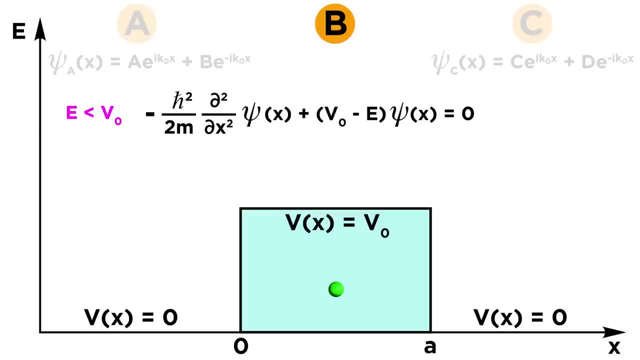 giving us the quantity V-naught minus E times psi of X. Now, from here, we will do almost the same thing as we have done so far. We will use a complex exponential. Let's multiply through by two M over H-bar squared, though, positive instead of negative. 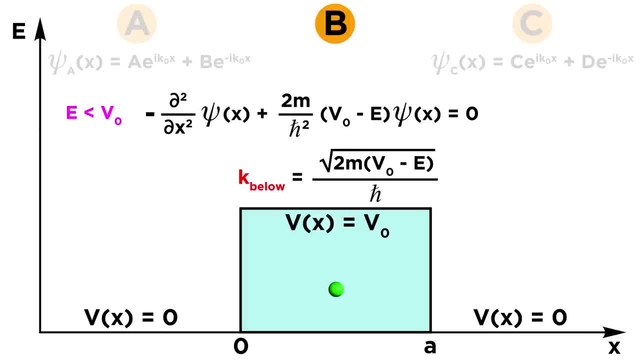 this time, and then define a K value, which this time can be called K below, referring to the set of energies that are below the barrier. This will be equal to root two M times the quantity V-naught minus E over H-bar. 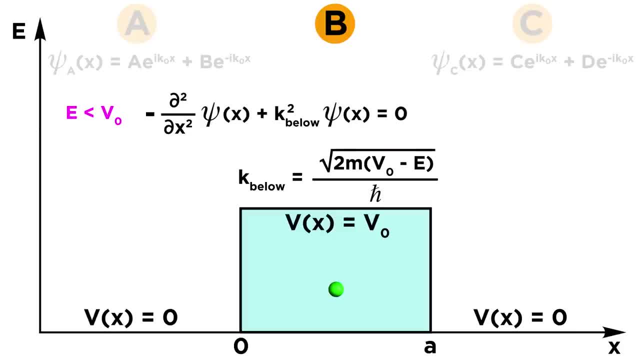 That means this whole term can be written as simply K below squared over H-bar. Now let's look at the next example. Let's look at the next example. Here we have U squared times psi of X, And with that substitution we have second order differential equation of precisely the 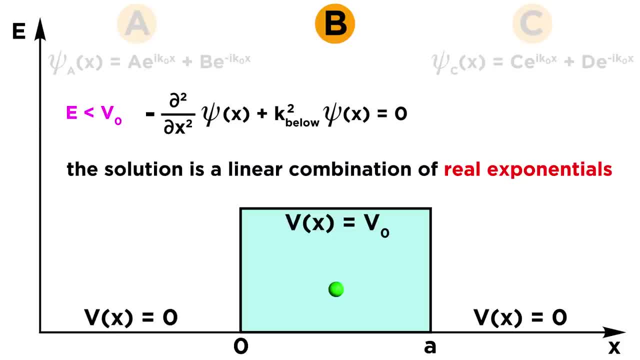 same form as we solved a moment ago. This means we can now write out our solution for the wavefunction as a linear combination of real exponentials. Since the constants A through D are taken, let's write this as: psi B below of X equals. 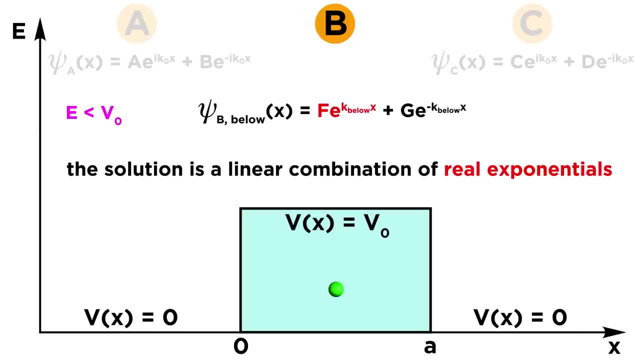 F times E to the quantity K below times X, x plus g times e to the quantity negative k below times x. Again, this is the only solution that will utilize real exponentials rather than complex exponentials, because it's the only region where the particle cannot travel freely. 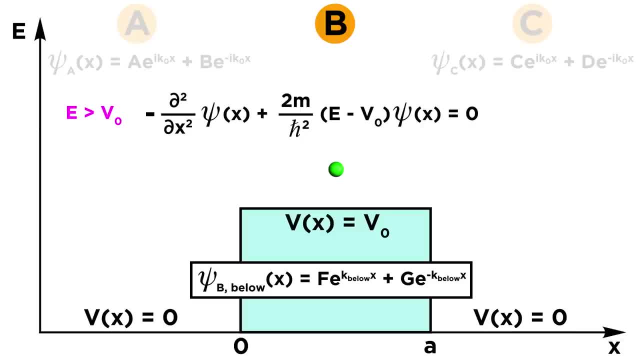 To finish this off, let's consider the case where e is greater than v-naught or higher than the height of the barrier. Here, everything will be the same as what we just saw, but let's use a different constant, k above, which is the same as k below, but instead. 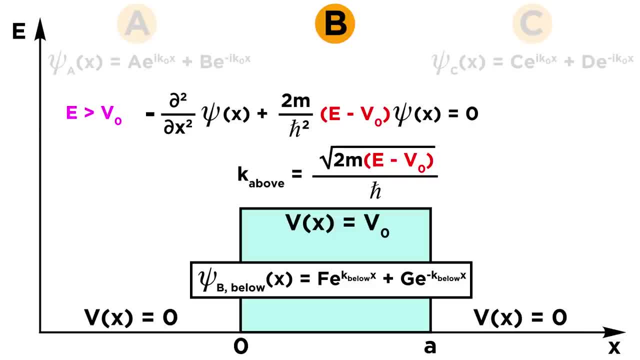 of v-naught minus e, we have e minus v-naught in the parenthetical. As we would expect, the resulting wavefunction that acts as a solution to this differential equation will be a combination of complex exponentials, just like in regions A and C. 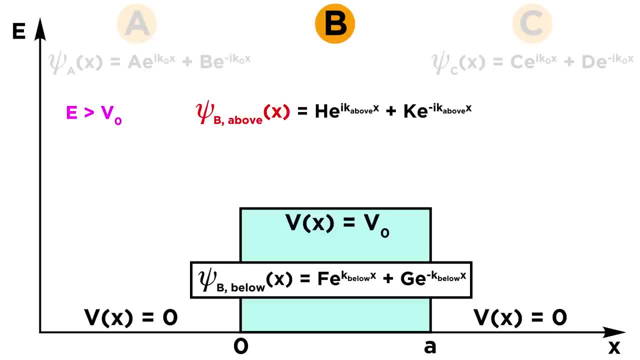 Requiring new constants. this can be written as: psi b above of x equals h-naught minus h times e to the i k above times plus k times e to the negative i k above times x. So just to reiterate what we did for region B of this diagram: we used real exponentials. 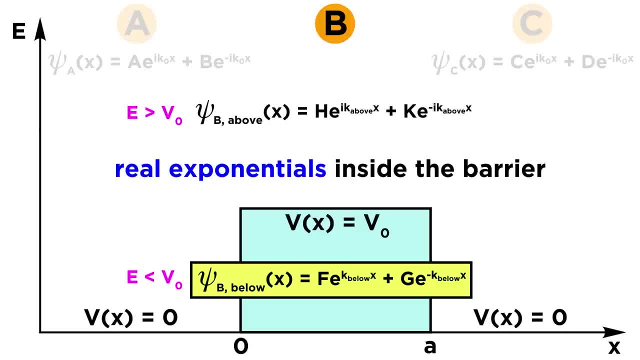 inside the barrier, because we expect a decay of the wavefunction and a low value for the probability density function, since this is a barrier. But above the barrier, we used complex exponentials, because here we expect xi k over 2.. 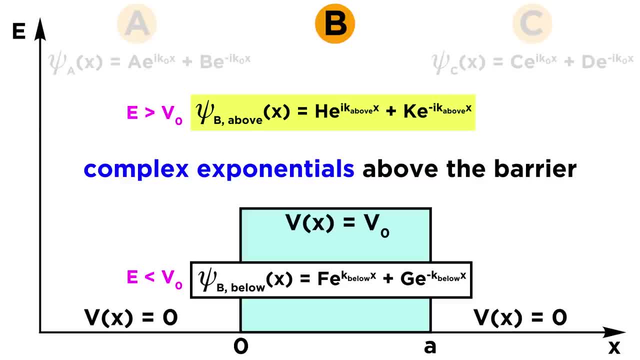 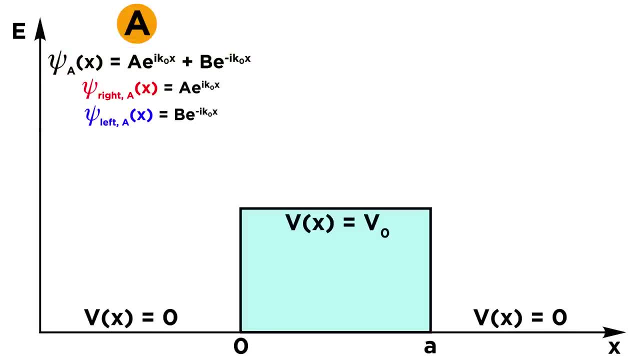 違 non-decaying wavefunction, just like in the other regions. So to synthesize everything we've done so far, this is the wavefunction for region A. Now let's split this up into psi right A and psi left A, which represent wavefunctions. 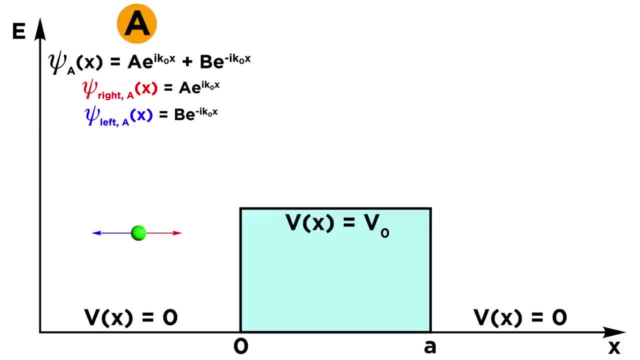 in region A, which have a part that may travel to the right and left respectively, where the coefficients A and B describe the relative probabilities of the particle traveling in those directions. So if B equals zero, there is zero probability of finding the particle traveling to the left. 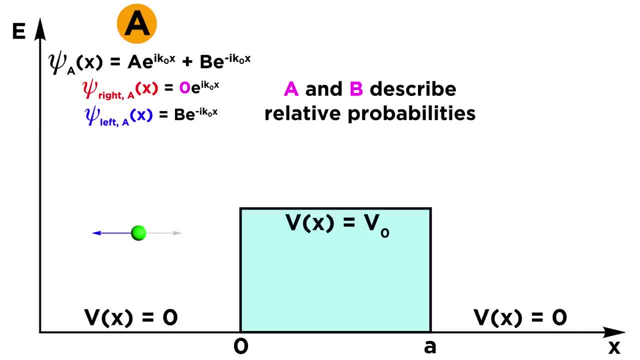 and if A is zero, there is zero probability of finding the particle traveling to the right. Illustrating the first example: mathematically we drop the B term from psi, A of X, because that term equals zero, and then write the probability density function psi times psi. 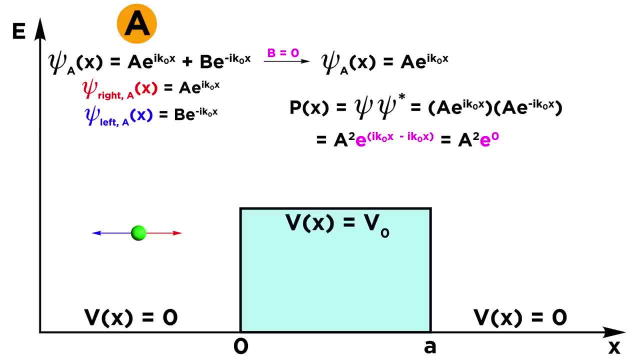 star, Because the complex exponentials multiply to give E to the zero or one, we say that we simply get A squared, which is the mathematical justification of why we can only find the particle traveling to the right. We can do the same thing for region C. Here we found this expression for psi C and we 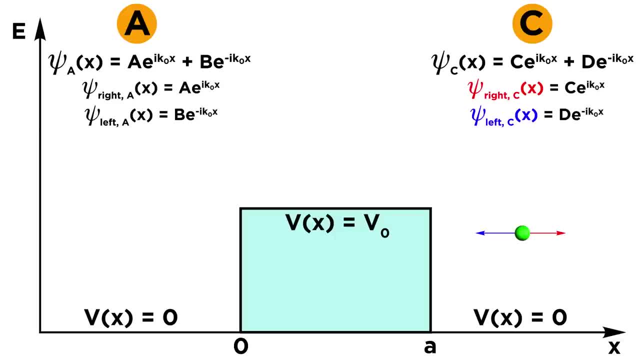 can split this up into psi right C and psi left C. And then finally, for region B, we found that the wavefunction will be different depending on the energy of the particle. For psi B below, we won't split this up into left and right, as they are all equal. 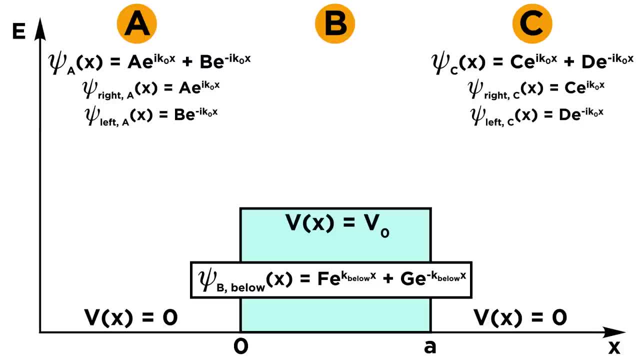 So we can split them up into psi right C and psi left C. And then, finally, for region B, we found that the wavefunction will be different depending on the energy of the particle. So we can split them up into left and right, as they are all equal and thus don't represent 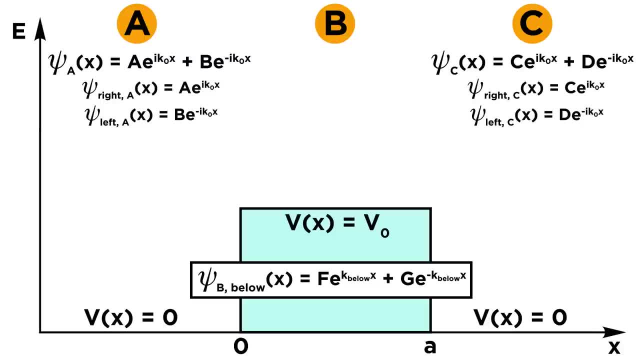 a traveling wave. In this scenario the particle is localized. But for psi B above we can again split this up and get psi B above right and psi B above left, just like we did for regions A and C. Now that we have everything set up, we are ready to find the solution. 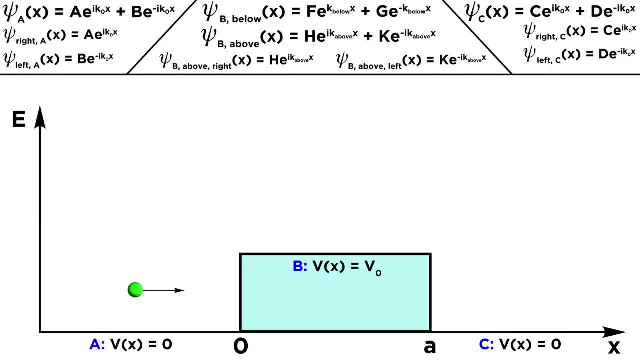 Let's consider a particle approaching the barrier from the left hand side. With this assumption, we can say that the current energy of the particle is equal to the current energy of the particle. constant D is zero. There can be no wave coming from the right side of the barrier and there 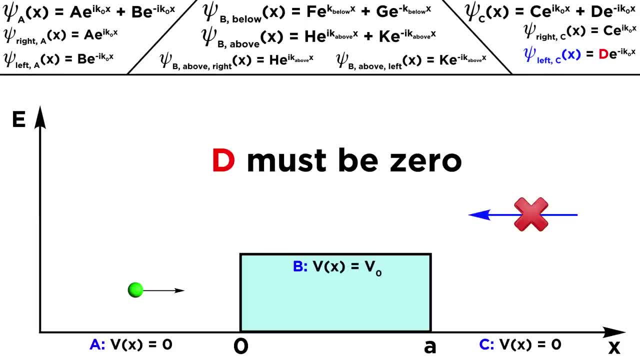 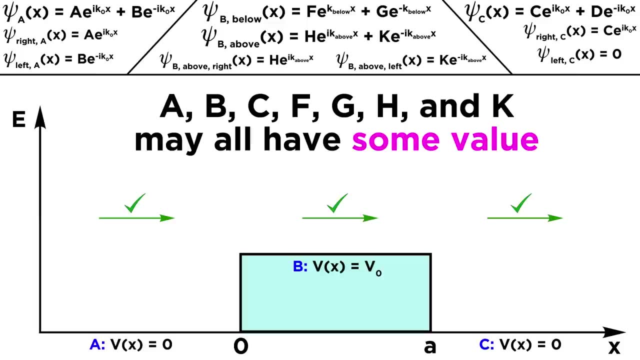 is no way for a wave traveling to the right to reflect once beyond the barrier and come back the other way. so this constant must be zero, Meaning that psi left C equals zero. All other constants may have some value, because motion to the right in A, B and C is implied. 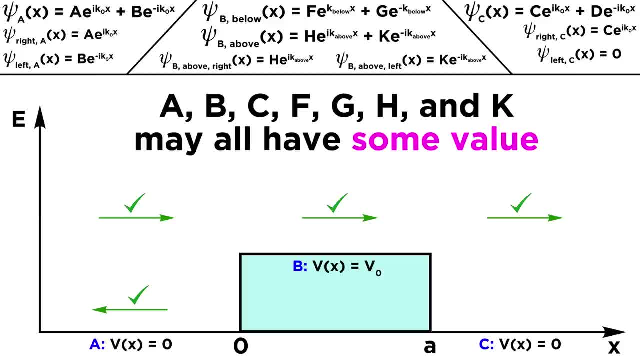 if the particle surpasses the barrier. Motion to the left in A occurs if the particle reflects, and even motion to the left in B is possible if the particle penetrates the barrier to some degree prior to reflection. So motion to the left in region C is the only motion. 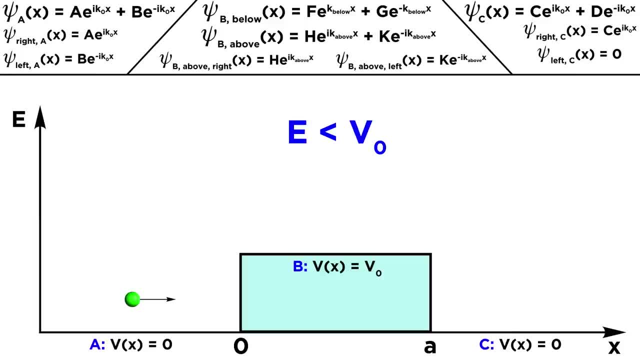 that is not permitted. So let's look at a particle with an energy that is smaller than V-naught by applying the boundary conditions to get the constants as well as the solution to the Schrodinger equation. So, just like with the particle in a box, we need to find the conditions under which. 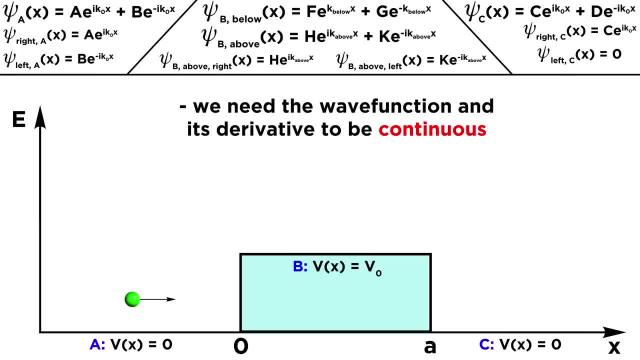 the wavefunction and its derivative are continuous over the spatial domain where our problem is defined. The wavefunction must also be normalizable, meaning that the integral over the relevant domain of the wavefunction times its conjugate must equal one. First let's examine the boundary. x equals zero. This is the boundary between regions. 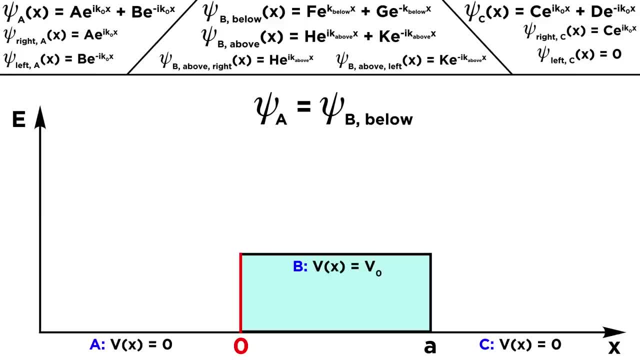 A and B, and at this position, we need for psi A to equal psi B below. By setting these equal to one another at the boundary, we are ensuring the continuity of the wavefunction over the boundary. Furthermore, we must ensure that the wavefunction is continuous at the 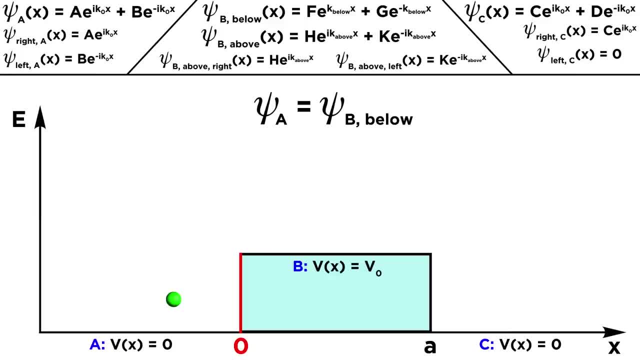 boundary with the barrier in a way that is independent of its energy, such that it describes both a particle surpassing the barrier and a particle being reflected by the barrier. Let's write this out. Let's write this out with the full expressions now, Since we are examining: x equals zero. 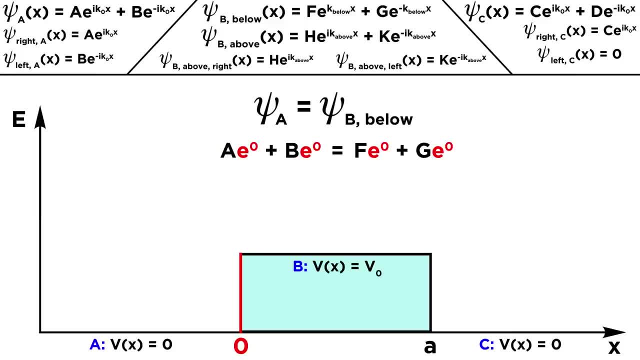 let's plug in zero. everywhere we see x. That makes all of these terms e to the zero and anything raised to the zero power is one. so that simplifies this significantly, leaving us with A plus B equals F plus G. Let's label this equation one. Now we also need: 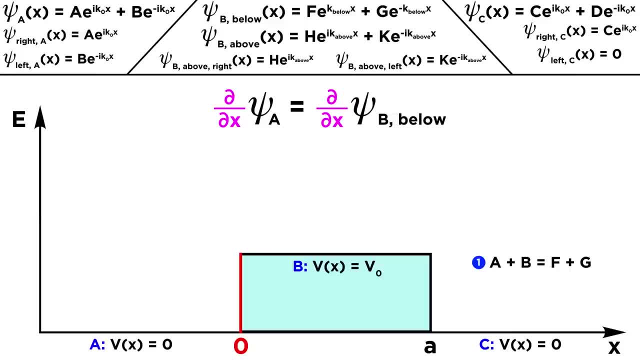 their derivatives to be equal at this boundary, because continuous functions must have continuous derivatives. This means that the partial derivative of psi A with respect to x must equal the partial derivative of psi B below with respect to x. Differentiating these expressions will be rather easy. we just pull whatever coefficients are in front of the x in the 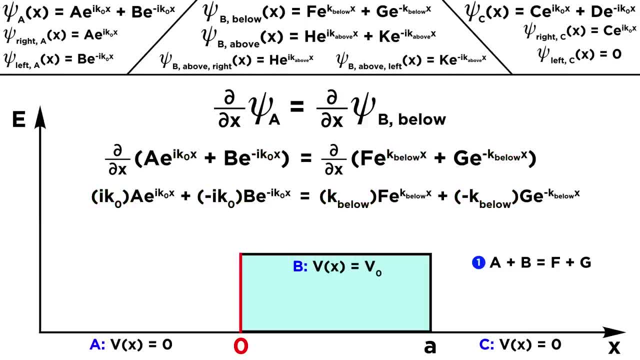 exponential terms out in front of each term, which leaves us with this expression. Again, we can plug in zero anywhere we see x, which makes all the e terms go away, leaving us with I k-naught A minus I k-naught B equals k below F minus k below G, And we can label. 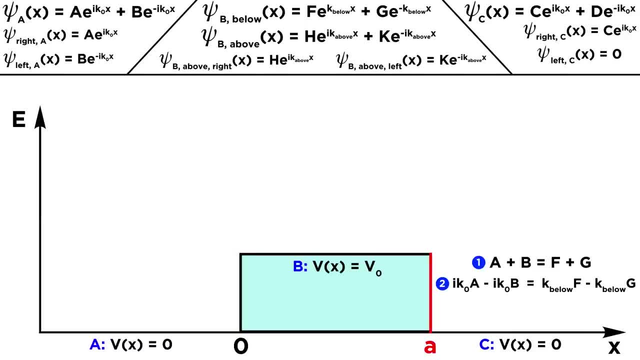 this equation two. Now let's examine the other boundary, the one between regions B and C, where x equals A. Here we need for psi B below to be equal to psi C again to ensure continuity for the wavefunction across this boundary. That will give us this expression. 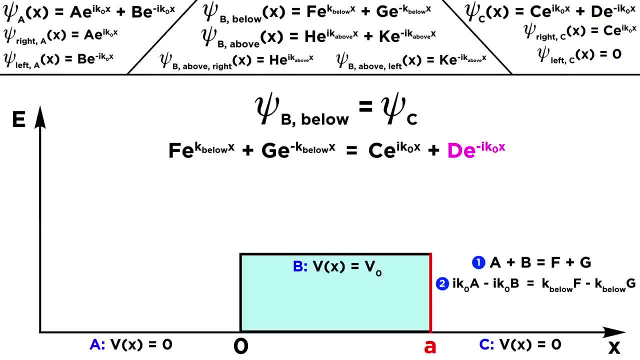 and recalling that we determined D to be zero earlier, we can get rid of this last term. Now, since this boundary has x equal to A, we can plug in A anywhere we see x. This time these terms won't go away, so we are left with this. Let's label this equation three. 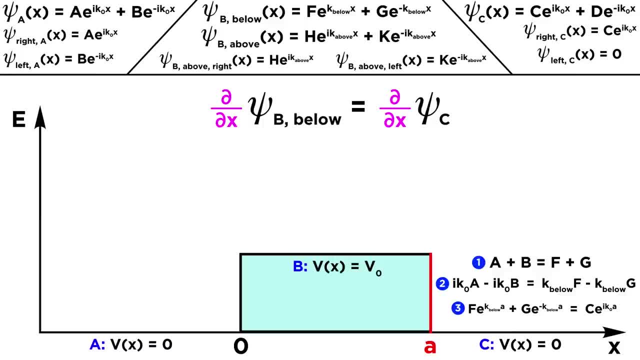 And finally, we need to find the conditions under which the derivatives of psi B below and psi C are continuous at x equals A. Take the derivative of this expression and then plug in A for x to get this. This will be equation four.